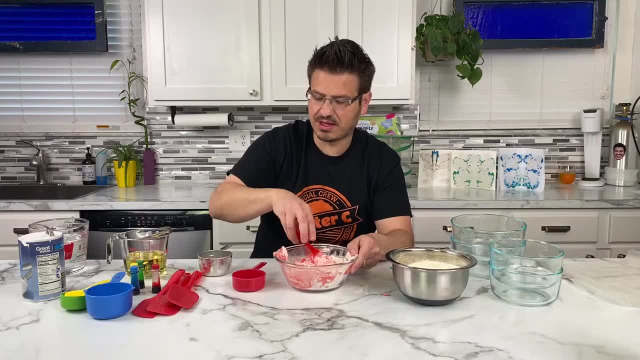 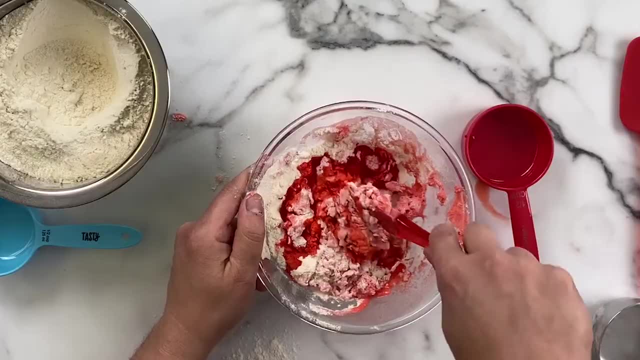 All right, so I definitely need a little bit more water. I think that's going to be a good little pink. Oh, it smells like flour. It makes me want to make pizza dough. Every time we play with the flour, I want to make pizza dough, All right, so 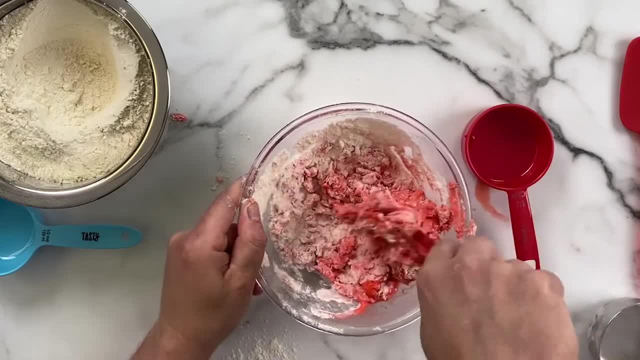 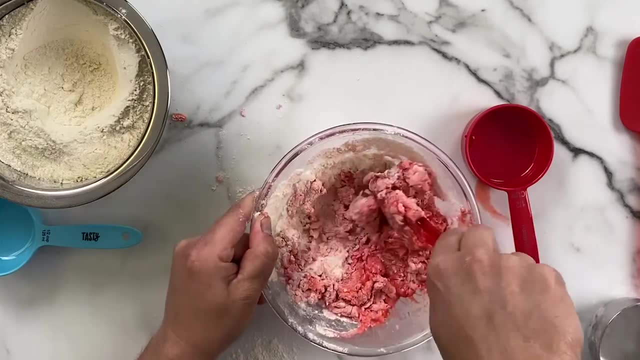 so I might need a little bit more water, But I'm going to, before I add more water, I'm going to work this a little bit and I'm going to pull it out and knead it. Oh, that's a good consistency right there. 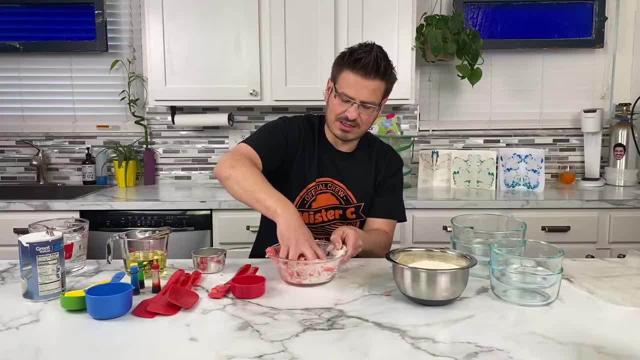 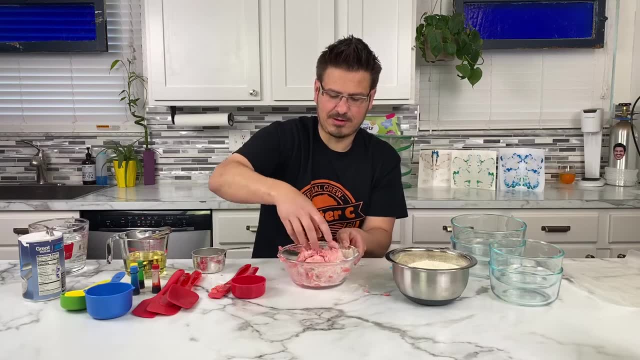 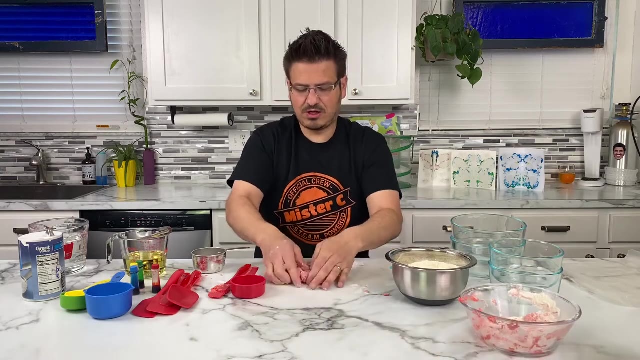 Yes, That's a good consistency right there. Yes, Yes, Yes, Yes, That's a good consistency right there. That's a good consistency right there. need it a little bit. I think sometimes it needs that. all right, this is actually pretty good consistency, so now I'm just going to. all right, it's crumbling a. 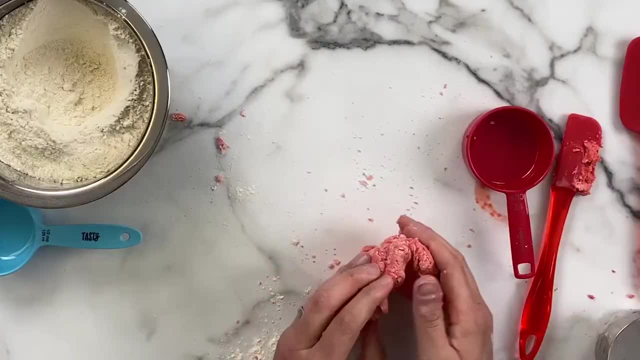 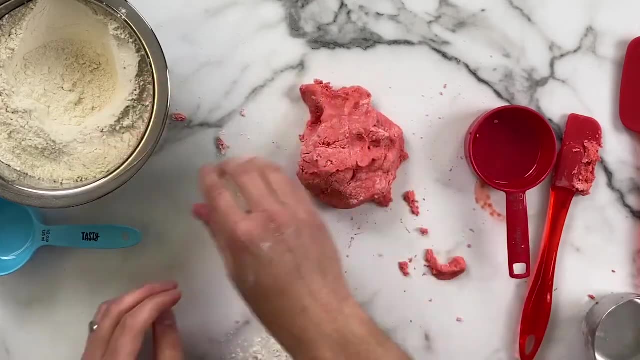 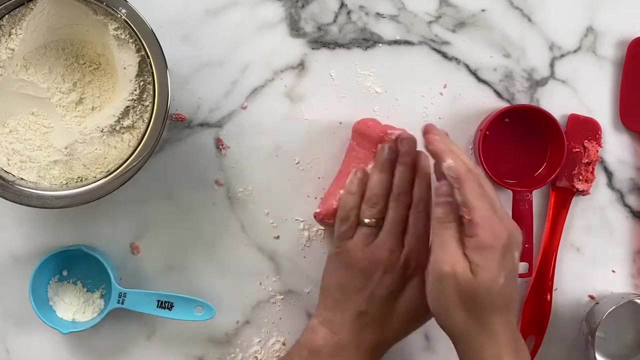 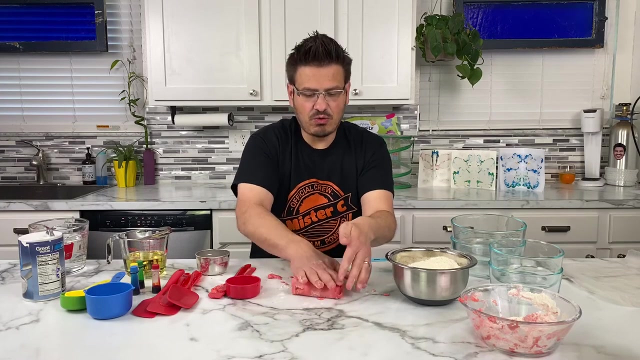 little bit. so it well, let's keep working it. now it feels dry, I'm gonna add a little bit of flour, but I'm gonna grab it. I don't put my pink hands in there, so if it feels like starting to feel a little sticky and you don't want it to, 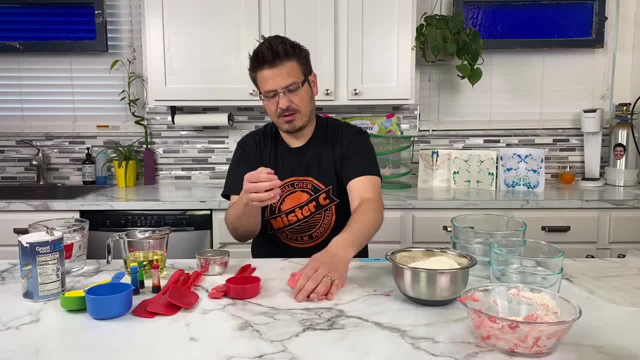 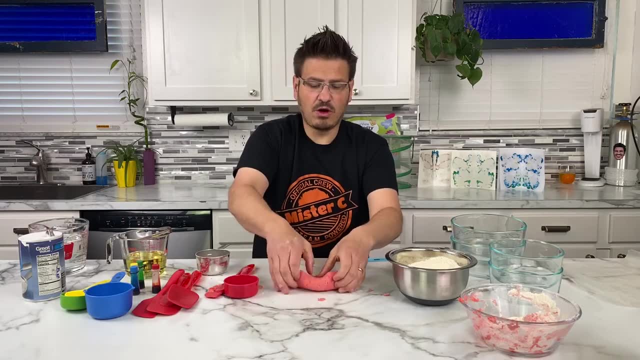 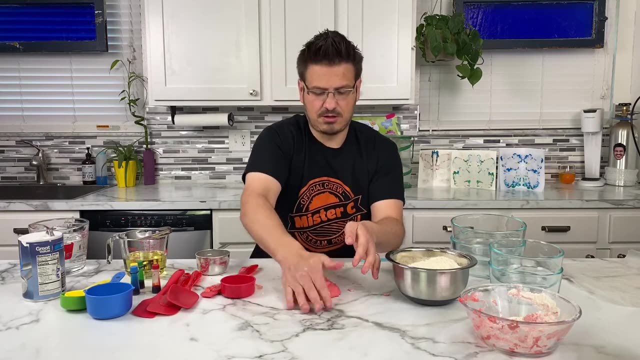 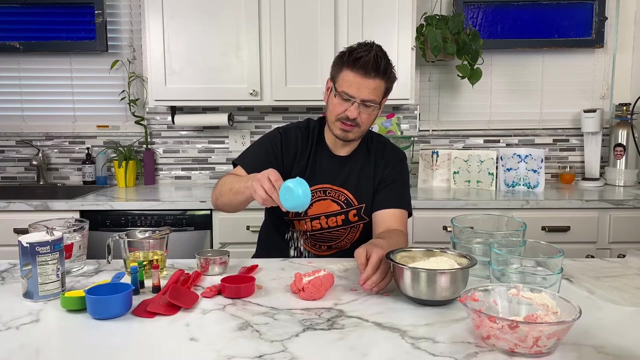 be, and so we're gonna add a little bit of flour. oh, this is really good consistency, though, and if you don't want to color, if you just want it to be like the, the whitish, grayish play-doh- yeah, I think that's a good pink. I'm not just a little bit more flour and it's. 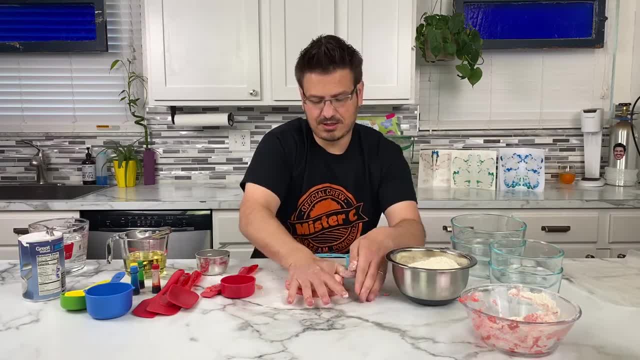 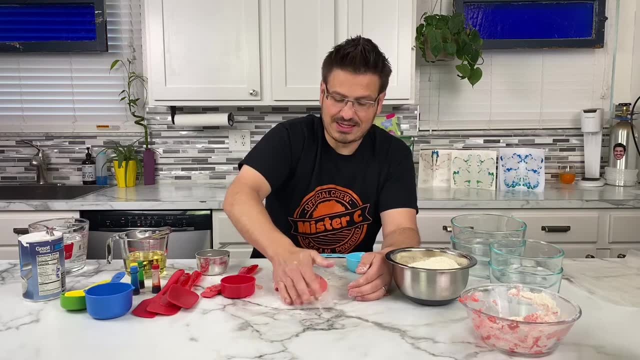 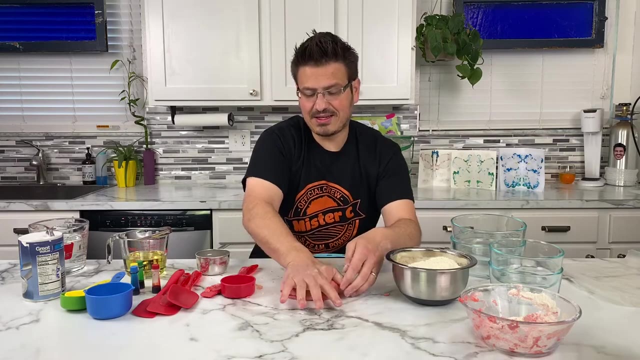 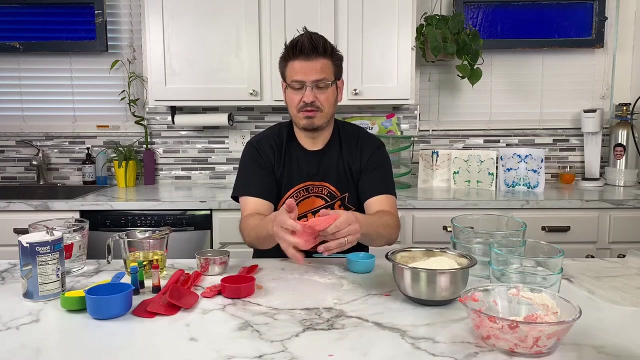 kind of where you want it to be in terms of texture. oh yeah, this is so cool. I love making this stuff because the best part about it is afterwards. you can make all sorts of shapes, designs, use numbers, letters, and really what I like is that for kids or adults who like to do things with their hands, it's a it's a it's. 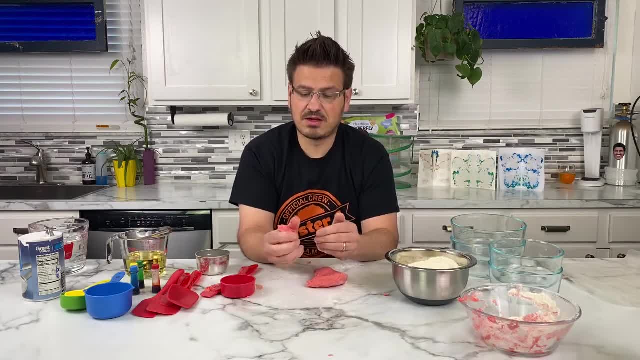 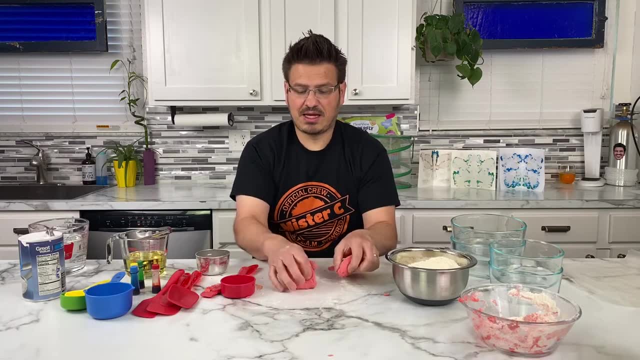 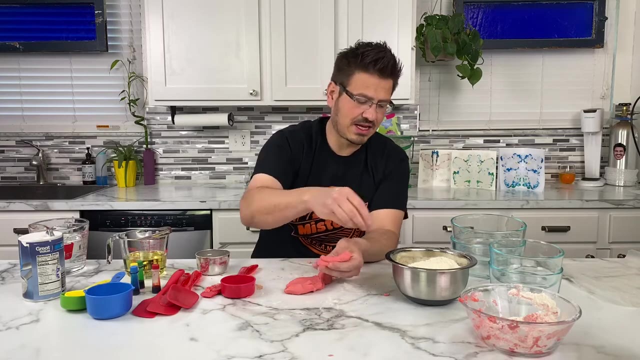 really high sensory. so for the preschool kids and parents and teachers watching, uh, they know exactly what I'm talking about and that's not just for little people, but like just texture and being able to um play with it. but yeah, I think it's pretty good. it's a little sticky on the inside, so I'm just going to break these up. 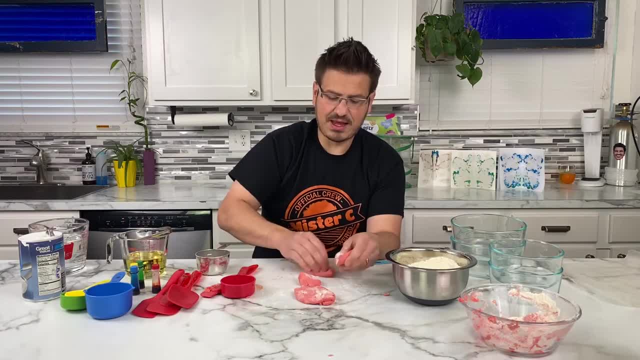 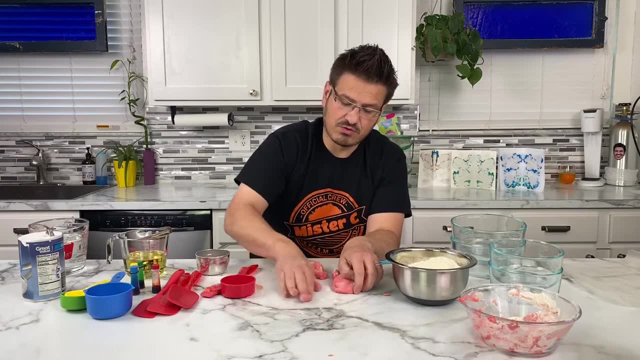 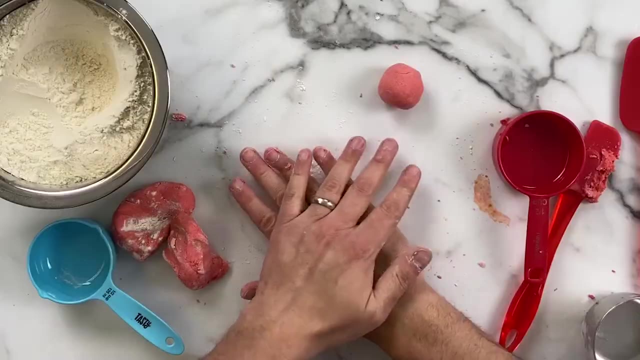 and you can keep playing and making this to the perfect consistency. so this is the salt recipe. I'm pretty happy with that. it feels good, and then you can roll it, make a sphere, or, if I want to work on my shapes, I can flatten it out. oh, I know what I want to make. 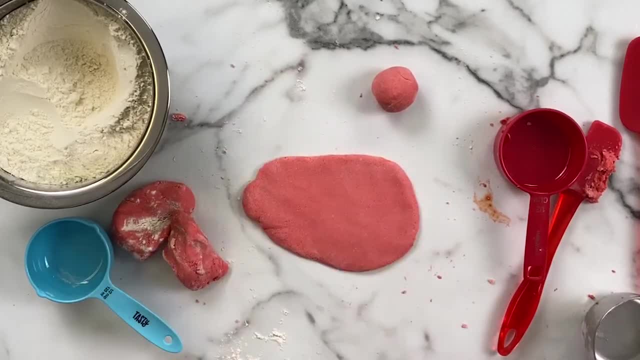 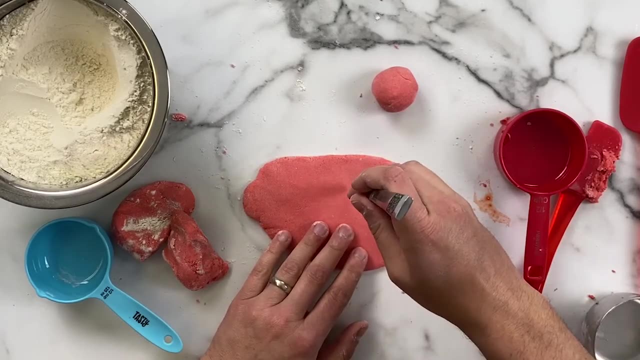 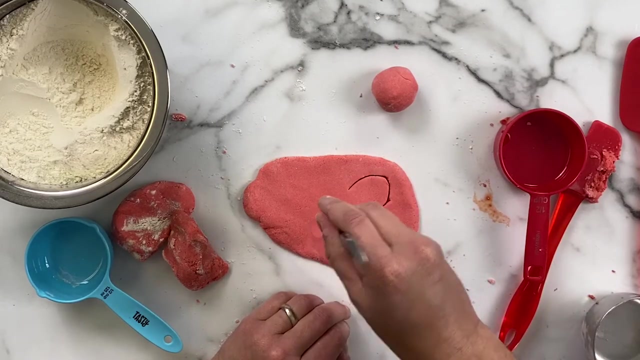 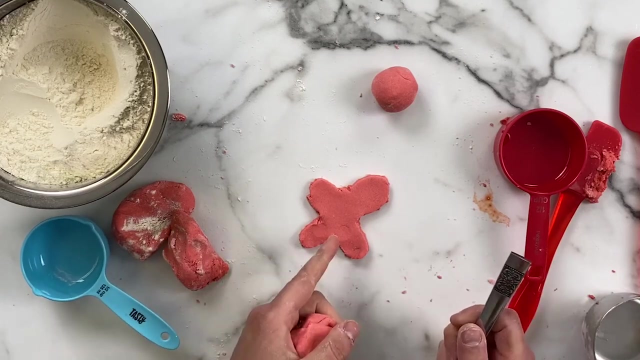 and you can let your imagination go wild. you can play, have fun. let's see if I can make. I don't know if I'll be able to make it, but we're gonna try it. I know what you're thinking: it's a plus sign, but it's a baby. it's a little baby. 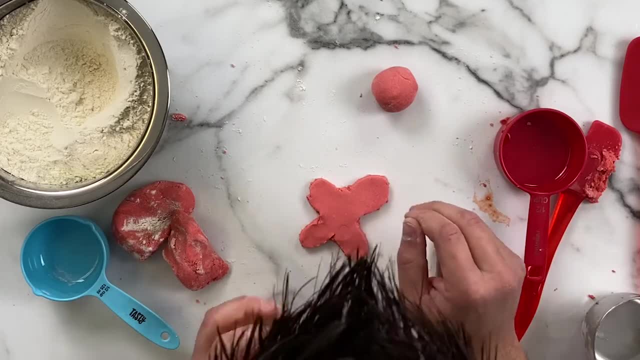 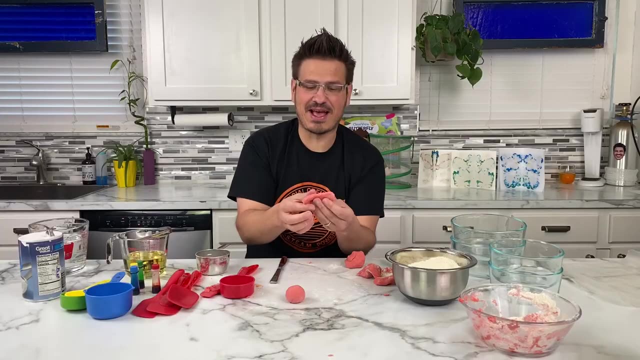 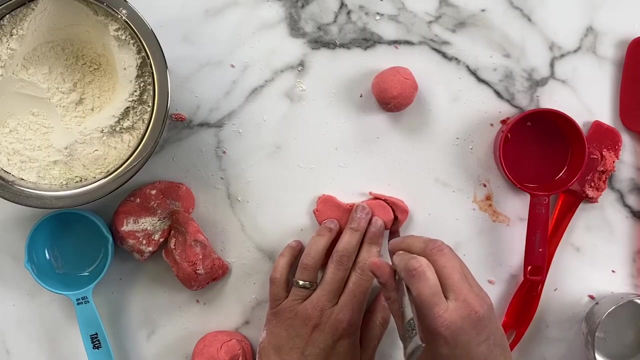 butterfly. my art skills have not been on the last couple of days. this matches perfectly with my design in the background. look at that, it's a butterfly. oh, this wing is just too big. it's not symmetrical, that's what it is. this wing is just too there. we go see. 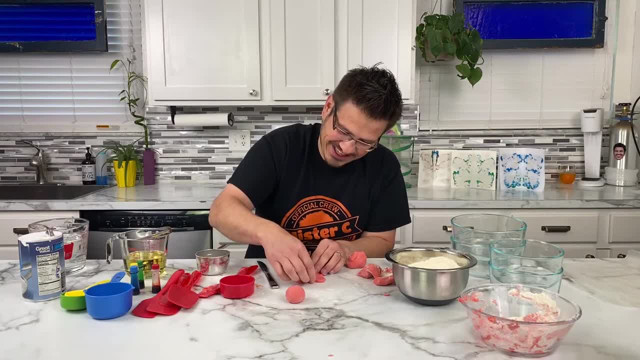 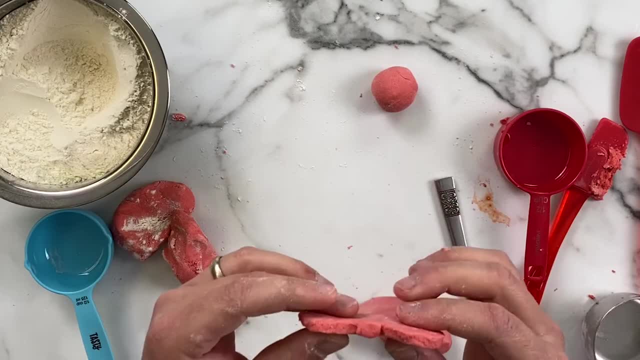 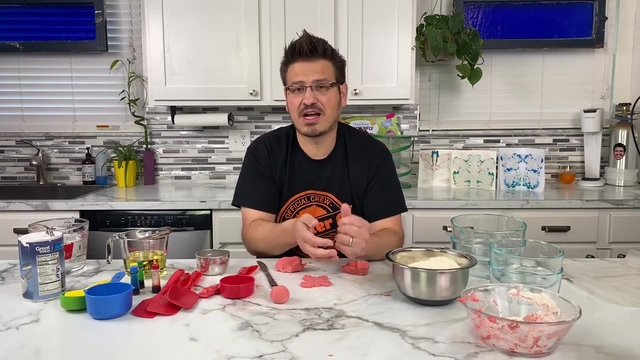 it does have a head. it's right here. there we go, there we go- perfect. it's like every butterfly I imagine making out of homemade Play-Doh. now you can do all sorts of cool designs. obviously you can do shapes, you can work on geometric shapes. so how do you build a sphere? 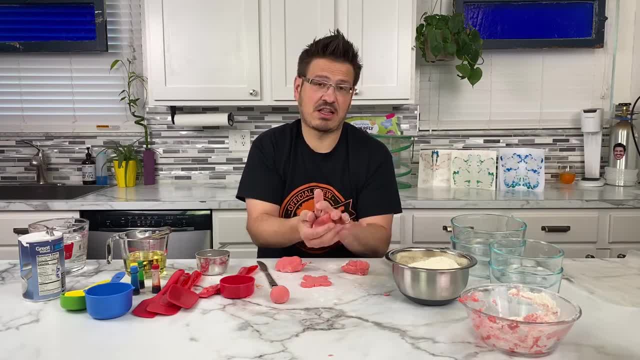 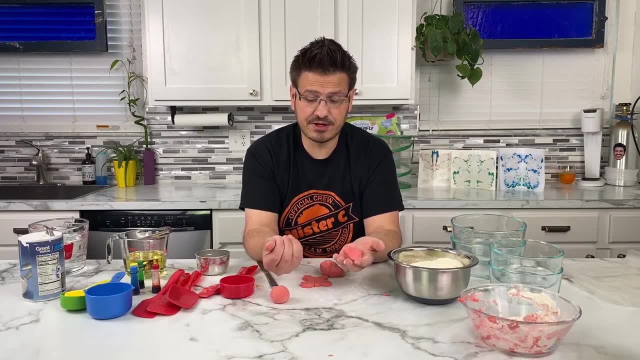 how do you build a pyramid, you know, turn it into something fun, a challenge for the family, and here's the really cool part. when you're done with this, my recommendation is to put it into the fridge in a Ziploc bag. it's going to hold longer. it'll hold probably three to four weeks, but because 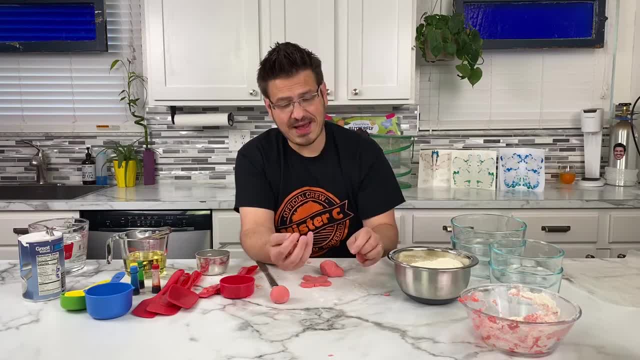 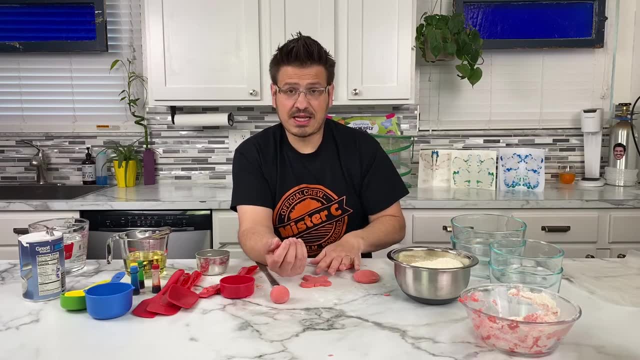 it's made out of flour and salt and water. eventually it's going to go bad. it's not like regular Play-Doh, but the more you can keep it cooled and keep it clean. so before you play with it, wash your hands. when you're done playing, wash your hands and then when you put it away. now here's the really cool.